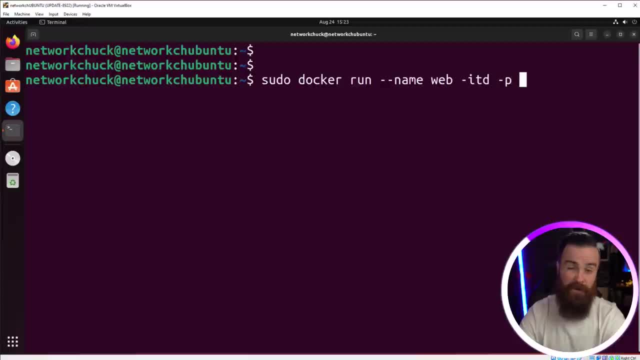 we'll name it web, do a few switches, ITD, expose some ports and we'll use Nginx as our image: Simple, elegant, the way our grandparents used to run it, but old. So what do you say? we do the. 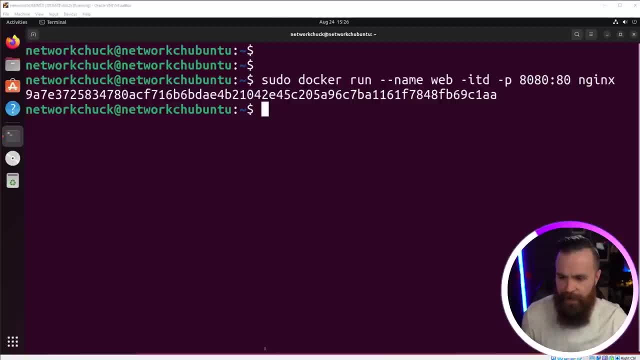 same thing, but with Docker Compose. So I'm going to skip through the process and I'm going to scoot this out of the way, but I'll keep it viewable right there And I'll launch another terminal Now. whenever you're working with Docker Compose, the first thing you want to do is make a 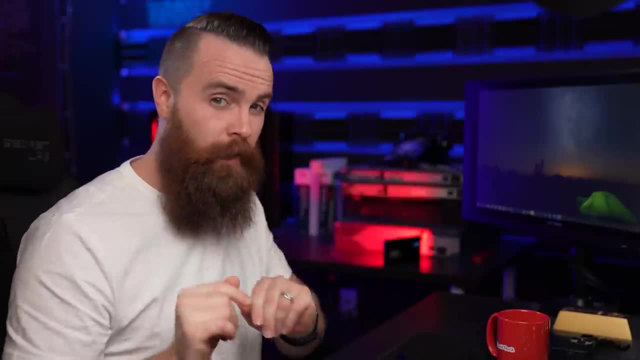 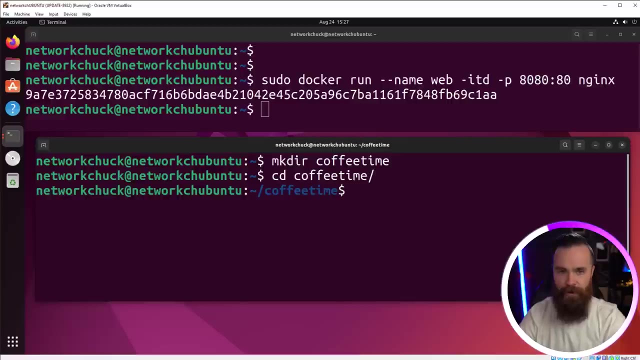 folder dedicated to that one Compose thing you're doing. It'll make sense why here in a second. So let's go ahead and do make dir and we'll name it coffee time, And then we'll jump in that directory- cd, coffee time. We're in And now let's make our Docker Compose file And it's just going to be. 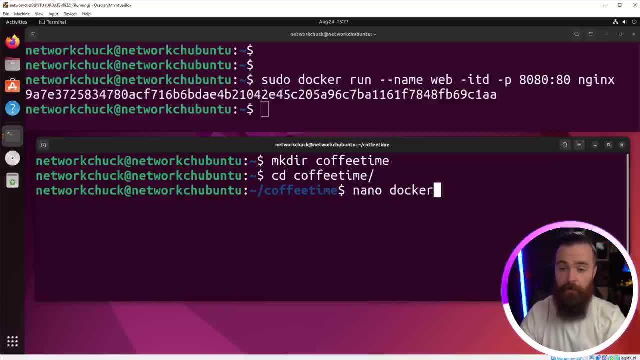 one file that does everything. It's kind of crazy. So nano docker-composeyaml. Two things here real quick. First, I'm naming it docker-composeyaml, Unless you have a really good reason not to go ahead and name it that When you're using. 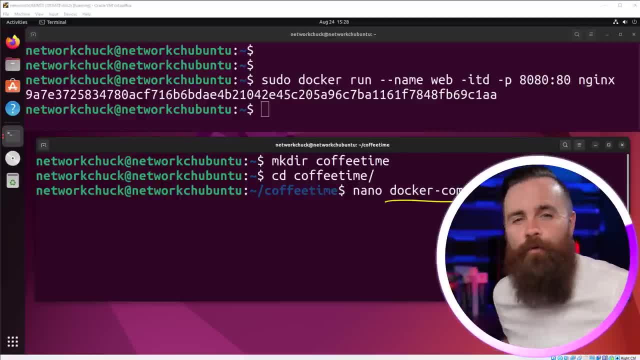 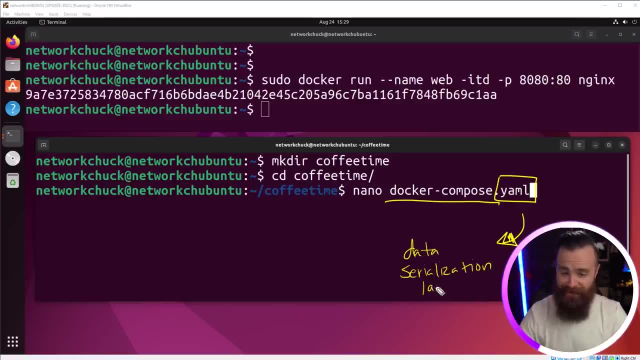 Docker Compose. it looks for that name by default, So why even go from that? Just do that. And then also notice we have the yaml, which is yaml. Technically it's a data serialization language, but that's too complicated. Just think about it as a configuration file. It's a nice. 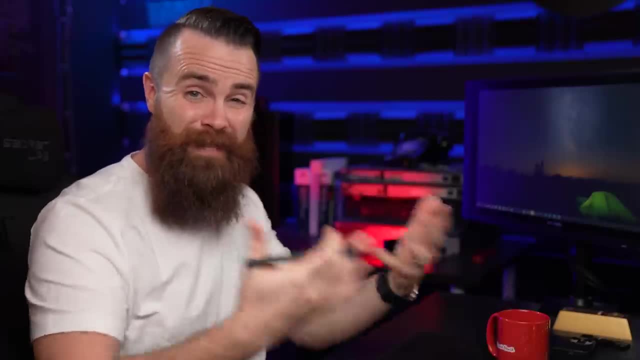 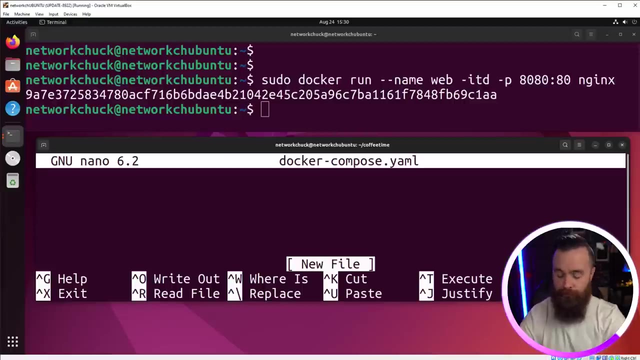 pretty way of writing out configuration. It's easy for computers to read and it's easy for us to read. You'll see it's beautiful. So let's go ahead and jump in that file, And here is where we'll start to write our symphony, our sweet, sweet Docker music. The first thing we'll do is: 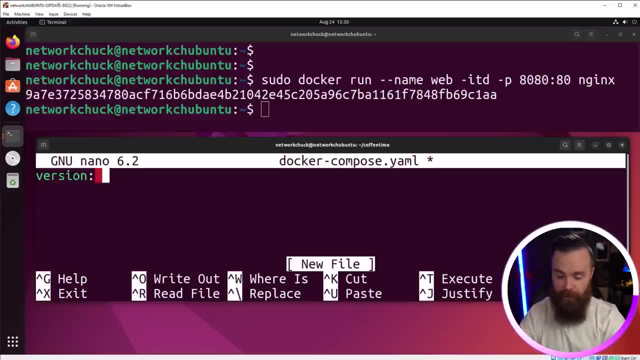 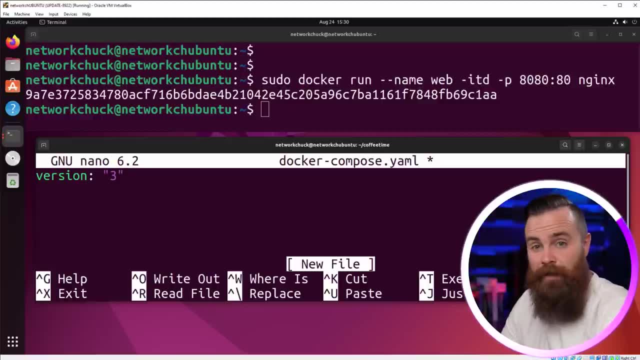 define the version by simply typing in version colon and then, right after that, putting in double quotes three. That's the current Docker version. You may be watching this in 20 years and we're at Docker version 12, 20.. I don't know, but it's three right now, So just do three Then. 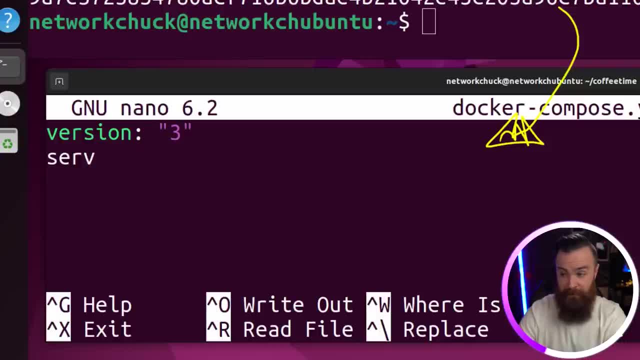 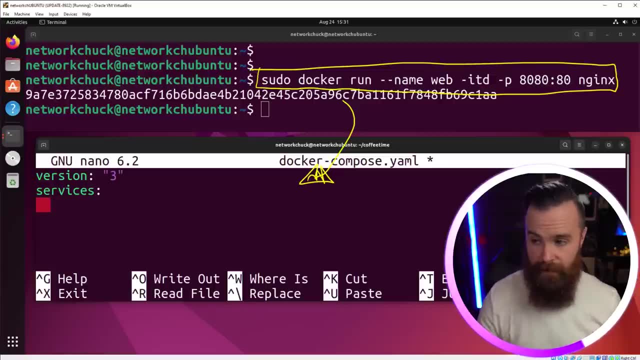 hit enter, Next we'll define services. So just type in services, if you can spell it right, unlike me. Hit enter and then tab. Now keep in mind YAML loves its space. It needs some personal space, just like Python. So when I say tab, I mean it Under. services is where we define. 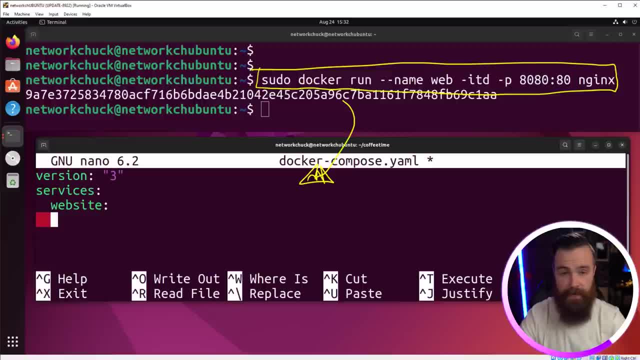 services. So let's call this guy website colon and then enter once more, And then I'll tab twice two tabs. and now I'll start configuring that container. First let's do our image Type in image colon. and what do we have? Nginx, That's it. So just type in Nginx, Get that part. 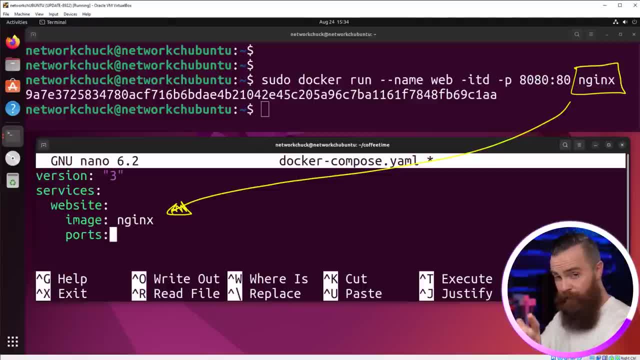 done And then right under there, keeping the same spacing, we'll do our ports, But watch what I do here. Again, this is YAML stuff, YAML speak. Tab, tab, tab. I'll do a dash space and in 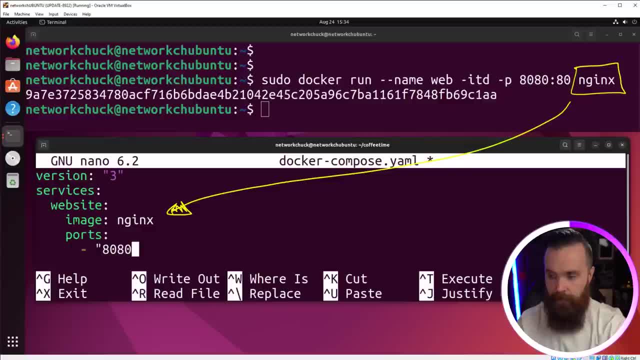 parentheses I'll specify the port mapping. So we're doing 8080, and actually we'll do 8081.. 8080 is already taken up right now and we'll map that to the 8080.. And then we'll do 8080,. 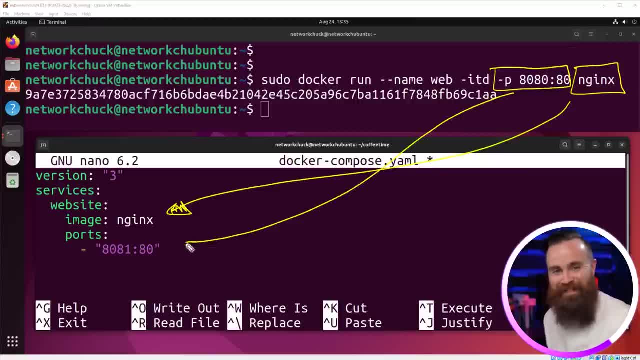 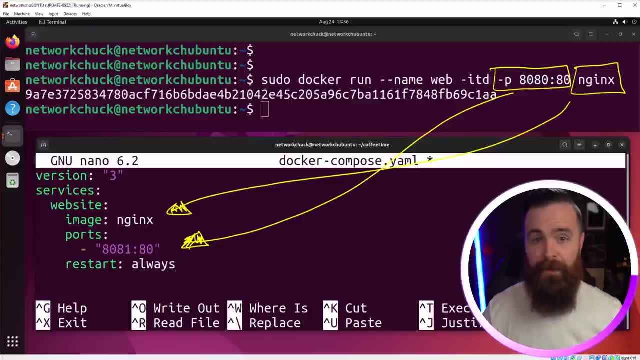 port 80 of our container. Now that is it, We're done. Oh, actually, there's one more thing we can do. Let's tab over to be in line with ports and we'll say: restart always. So it always comes back. 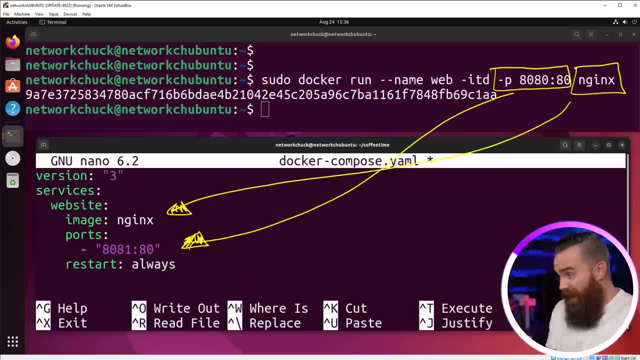 up after your machine reboots. You want that, right? Yes, Okay, So that's a Compose file, Simple, but it'll work. So let's actually try it out. I'll do a control. X, Y, enter to save. 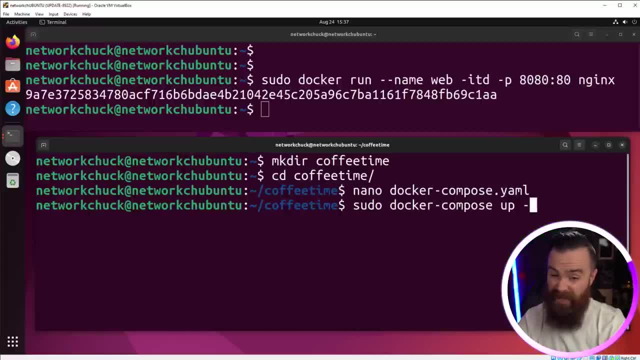 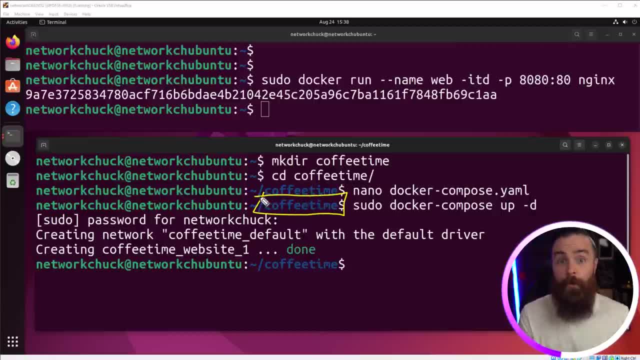 that command, while in that coffee time directory, the same directory where my Compose file lives. Make sure you do that. If you don't, you'll have to do some dash F and specify where it's going to. it's just a whole thing. Just make sure you're in the same directory. Also, notice this, Yeah. 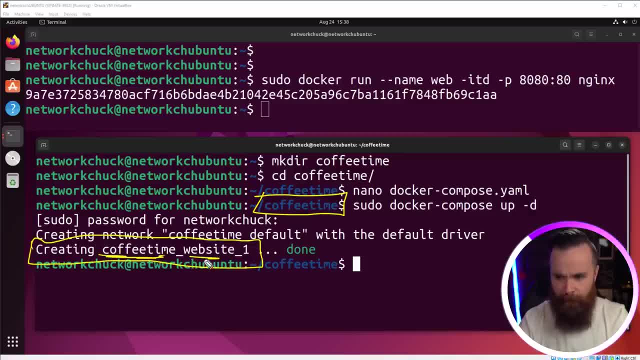 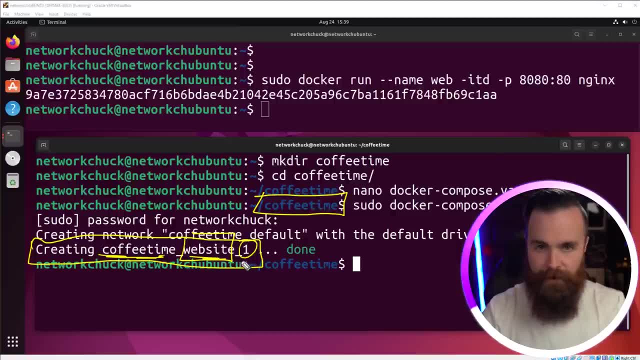 it did create my website, It named it coffee time underscore website, one which- coffee time- was the name of my folder, So that's why that's kind of important. And then, the website being the name of my service, And then it just puts one after it, like assuming you're going to make more of them. 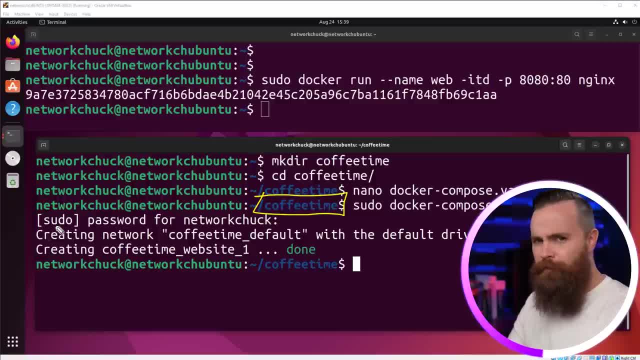 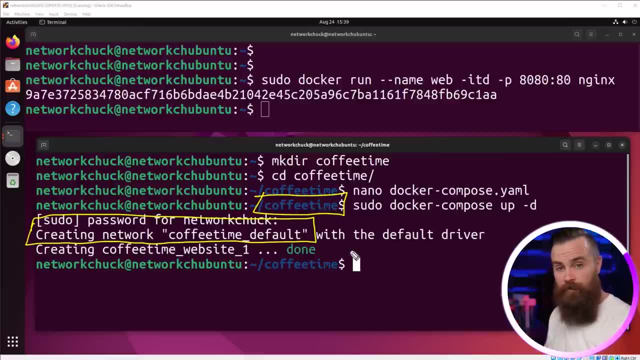 But then also notice: good old docker compose made a network for us too. That's some service. He created a default bridge network and put our container inside. What a good guy. And yes, that is the default behavior of docker compose, because we didn't do anything differently. You. 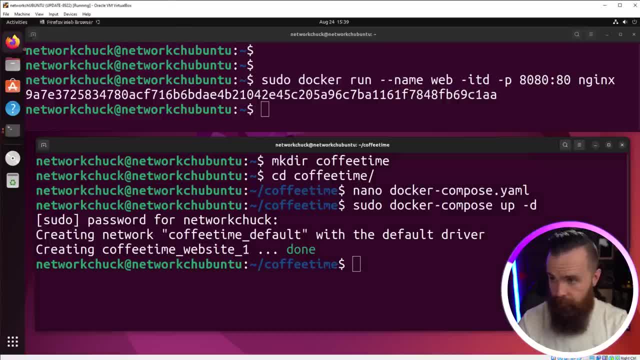 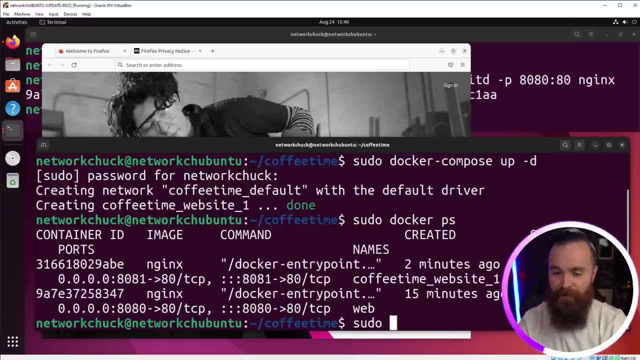 can change that and I'll show you here in a bit. Now I do want to make sure our website works. Let's go out there. Actually, first we'll do a docker PS. There's our two containers and there's 8081 right there, The one we just spun up And actually here. this is kind of cool If we do. 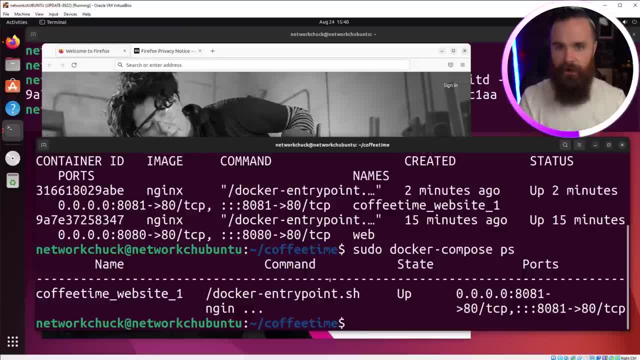 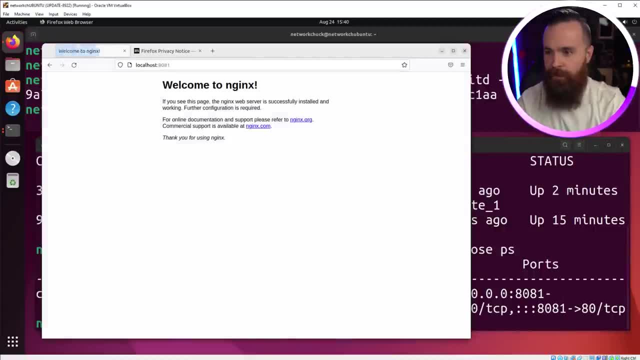 docker compose PS. it'll only show us the docker containers within that composed environment right there. That's kind of cool, And let's make sure things work. Local host port 8081, beautiful. Now, like I showed you in the intro, we can bring down that entire thing with one. 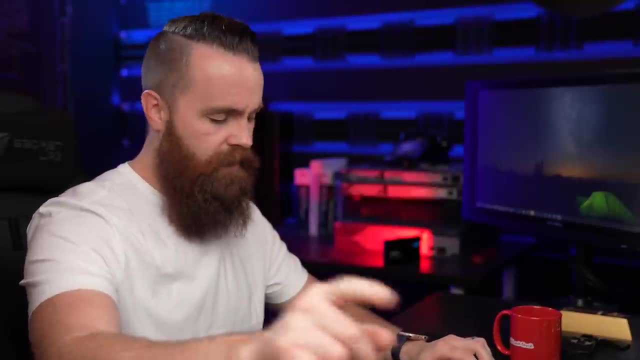 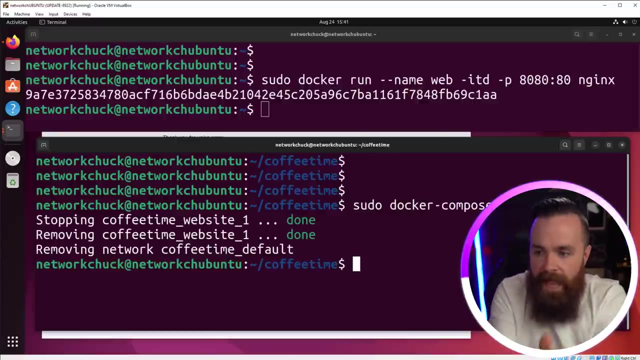 command and the entire thing. We have one thing in there right now. We're going to add more. just hang tight. but we can do pseudo docker, compose down, down boy And it just it deletes. In fact they removed the network and the container. Now we don't have to do that If 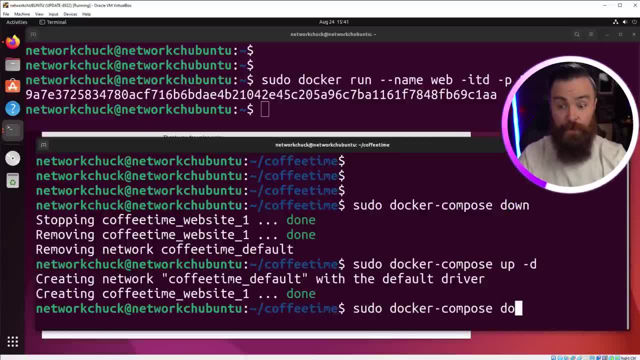 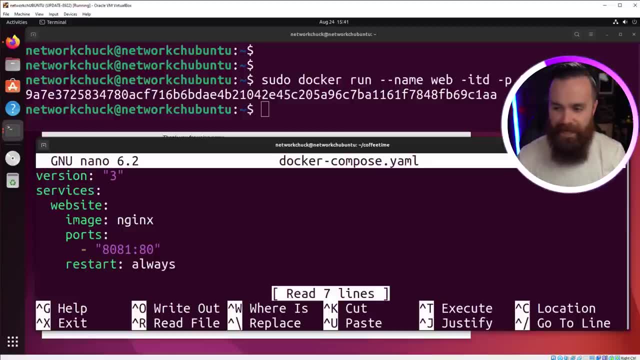 we just do another up command here. bring him back up instead of down. we can do stop, just simply stop in the containers. So you have options. I want to do down once more, just to delete it. So what I want to hit home here right now is that the docker compose file is: 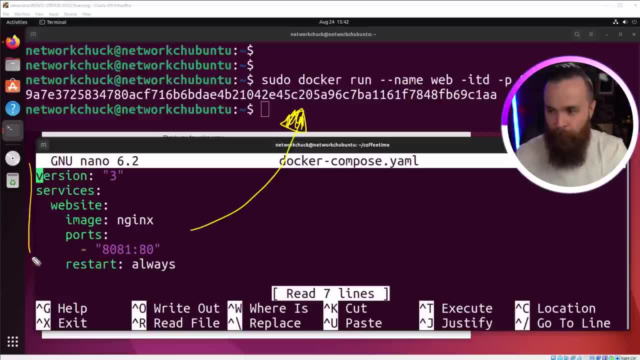 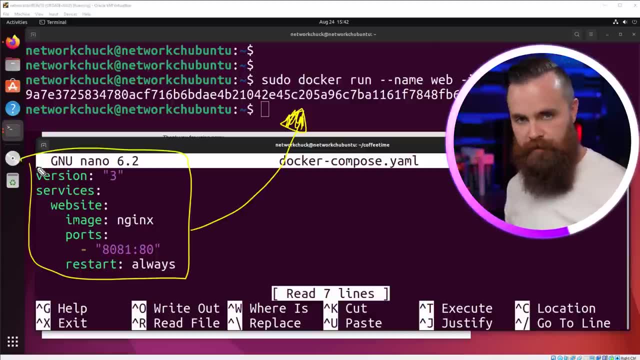 really the docker run command. It just looks a little weird. It has a different format. We have to describe it in a certain way, but that's really not too difficult with the power of Google. Just go look at some docker documentation. We covered the basics here, but there's obviously 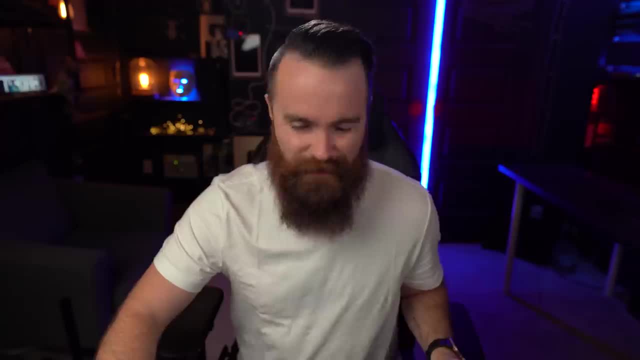 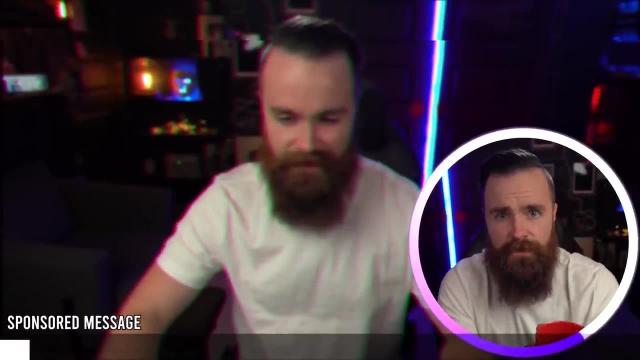 a lot more. So go Google it. It's pretty cool. but don't do it yet. I'm going to show you some more stuff, because we're about to get a little crazy Now. you know what I love about docker containers: They're safe, They're secure, They're isolated most of the time, giving you a bit of 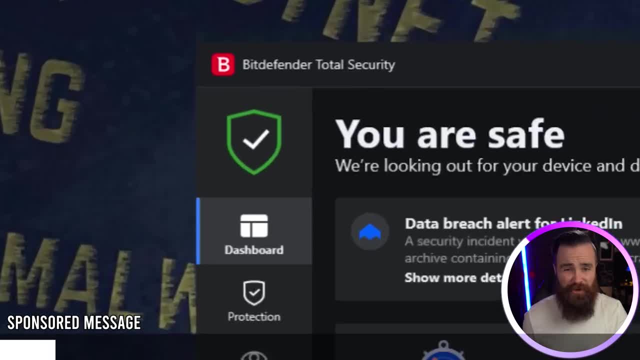 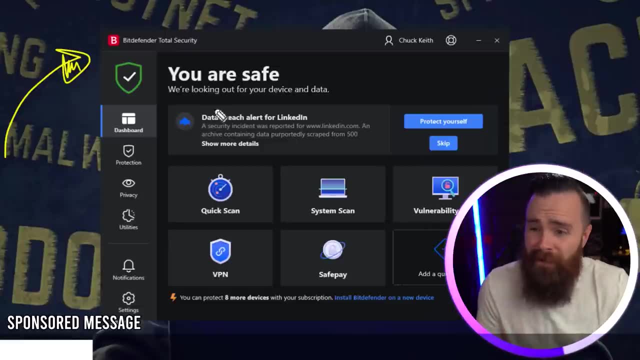 security. but you know what's not safe. you, your computer, because you're not using bit defender, total security. you're not living life inside of a docker container. You need protection. You need someone to hold you and tell you that you're safe and that they're looking out for you. and 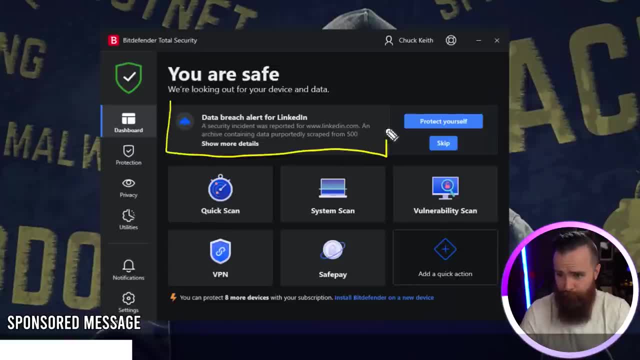 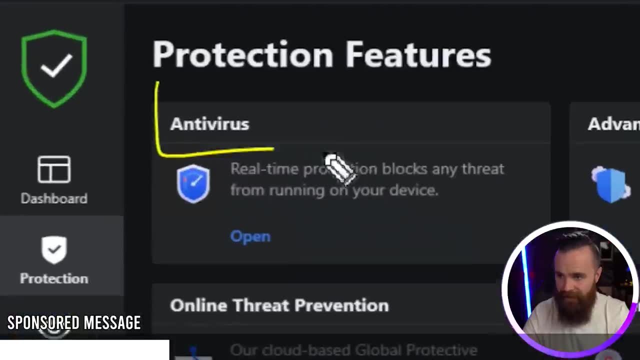 your device and your data and shoot. Look at that. This is new data breach alert for LinkedIn. Are you on LinkedIn? Well, there you go. Bit defender has our backs for protection. They got you with the antivirus advanced threat defense. They're also doing some crazy online threat prevention. 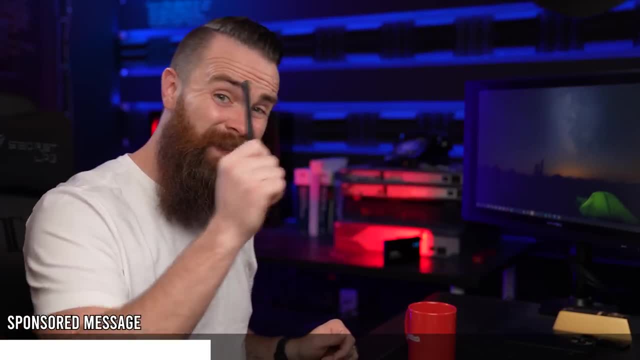 They're doing some cloud-based magic by blocking online threats at the network level And, should anything get through- which I doubt it- they're going to be scanning Your system for vulnerabilities, but it's not getting through because they get a firewall going. on. It's crazy. And then I know many of you wish you would have had this before it was too late. Ransomware remediation: They'll help restore your encrypted files If you get hacked. and no, don't just assume you're safe, Don't just assume you're immune. Anyone can be hacked, Even me. 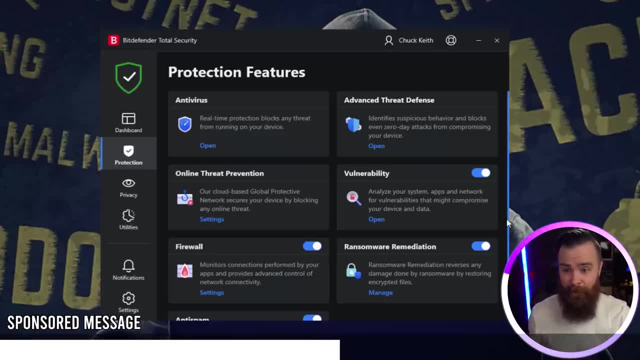 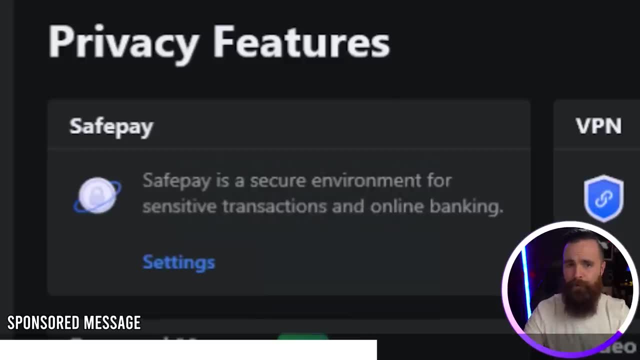 That's why I had this And one of the biggest ways you can be hacked. This is why I have my employees use this phishing attempts. I think it's an anti-spam going on And I know my audience. I know you guys care about privacy, but defender premium security has your back with safe pay. 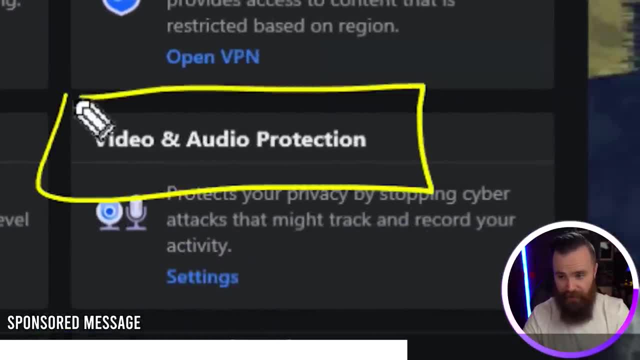 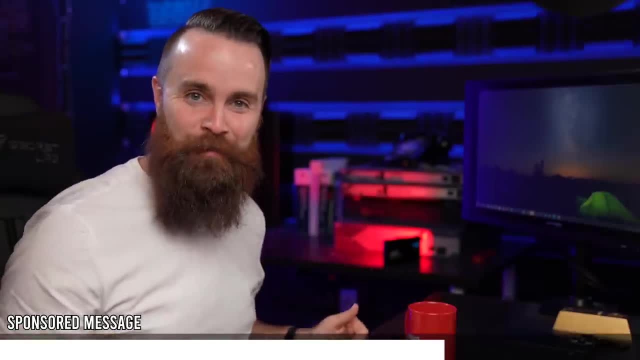 VPN password manager- And this is pretty cool- video and audio protection. You're always wondering: Hey, is someone listening to me? Can they see me on my webcam right now? They'll make sure they're not. they'll have that control in place and they'll make sure no one's tracking. 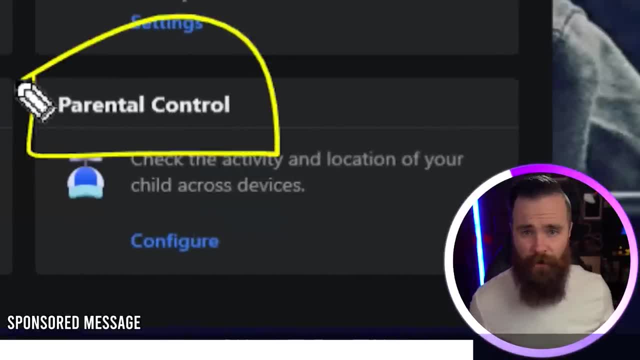 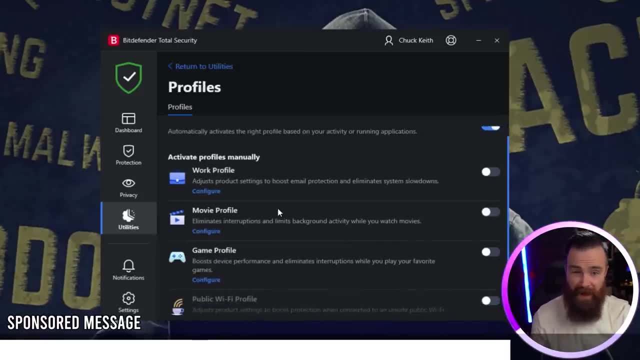 you and they'll make sure. Hey, are your kids being a little crazy? Cause mine are always being crazy. to help me keep track of my kids And you don't have to worry about performance with bit defenders profiles, You can tell them: Hey, right now I'm working, or Hey. 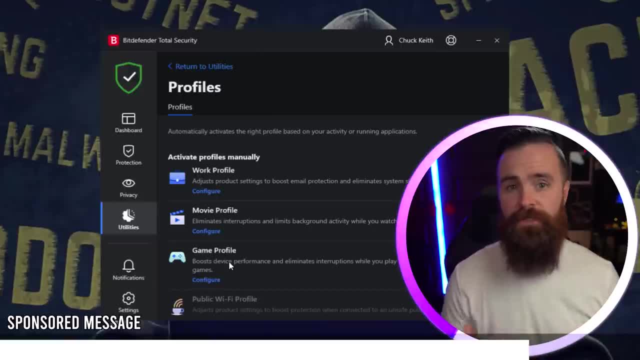 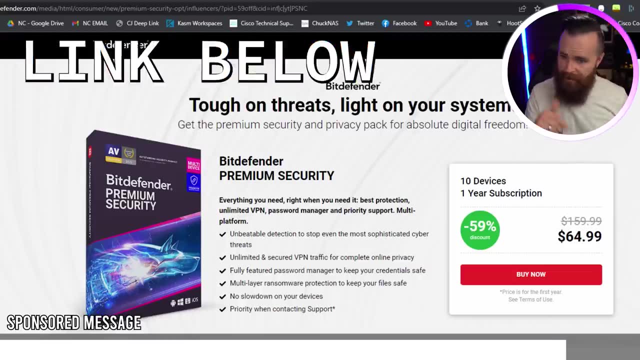 I'm playing a game. Please don't bog down my system. They'll adjust to what you're doing at the moment, So you can toggle that yourself or just let them decide. They probably know better than you. So check out. bit defender- premium security. I got a link below. 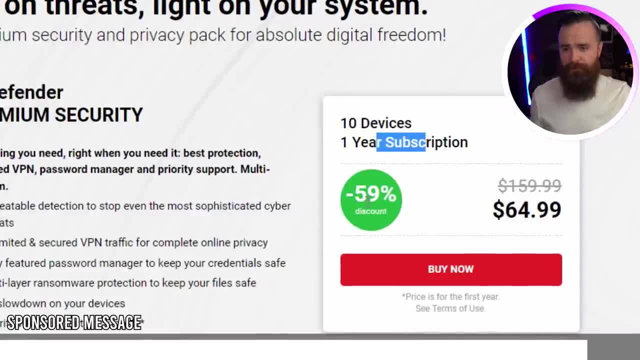 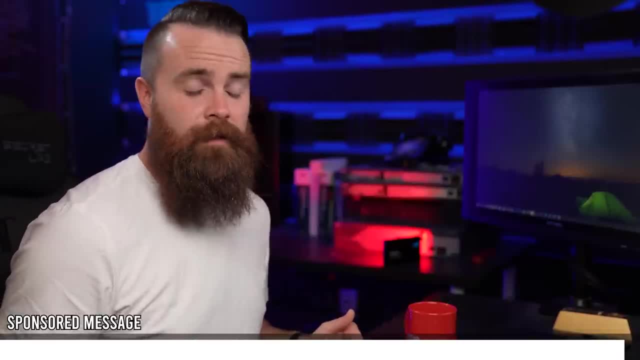 It looks like they're giving us dad gum: 10 devices, one year subscription and 59% discount. Don't miss that, because again, we don't live in Docker containers, even though that does sound kind of awesome, We don't. So back to Docker compose. with our compose file we can create: 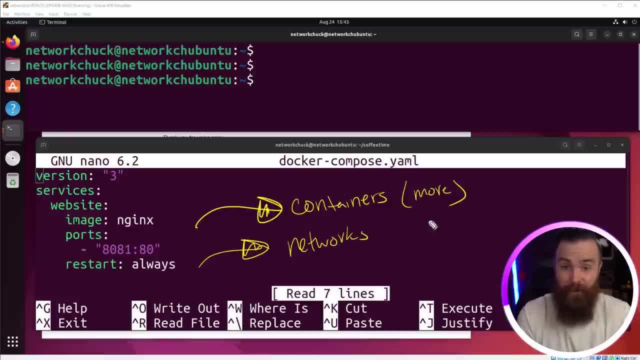 just a ton of containers, Like I mentioned before, inside and also we can create networks. So real quick, let's add another container, Let's just do a duplicate of our engine X container here. It's gonna copy website here And then making sure. 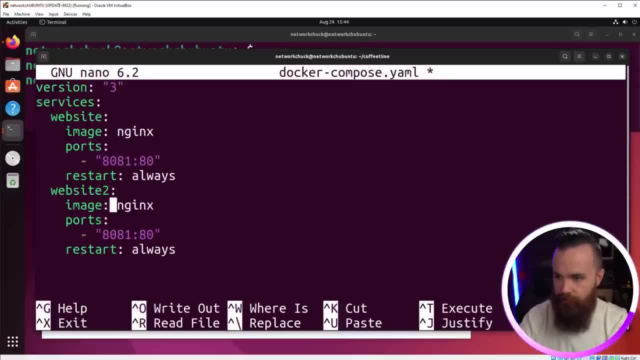 direct spacing. I'll paste it right there And I'll just rename a few things. Website too, We'll do a different port 80, 82 this time, And noticing that I'm keeping both these containers under the services section. And now we have two containers: control X, Y, enter to save Docker, compose up dash. 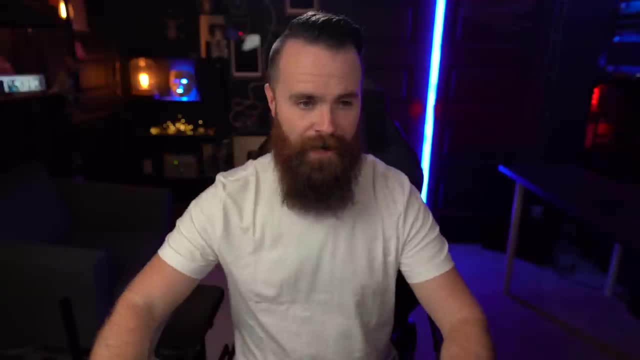 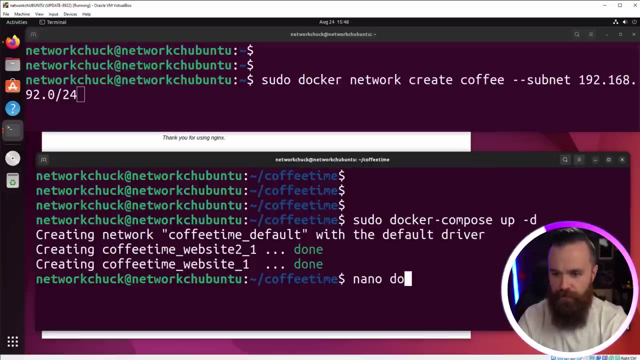 D, two containers. but we're not stopping there. Let's add a network. Now. if you watch my Docker networking video, you can watch that right here. Normally, to create a network, you have to run a command like this: Let's do the same thing inside a Docker compose file, nano. Docker compose dot. 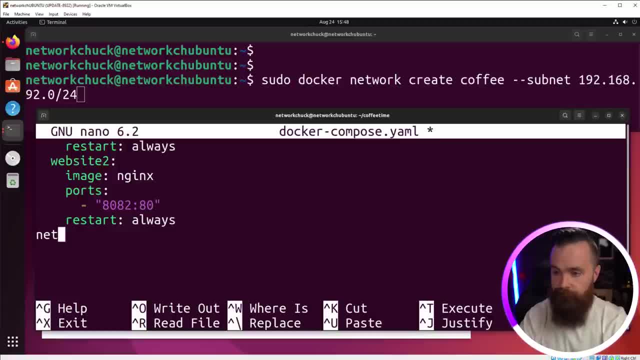 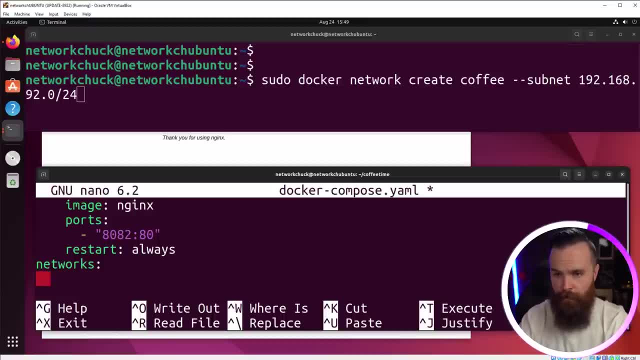 YAML And down here underneath our containers, we'll start a brand new section called networks, Noticing that it will be in line with services. It's a top level config and then we'll tab over name our new network. It was coffee, right, So we'll do coffee. colon. enter tab, tab. 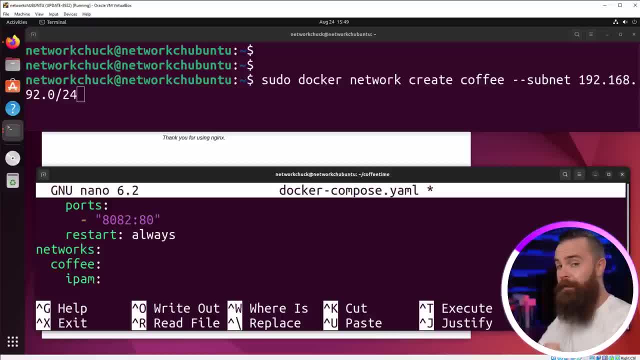 here It does get a bit different. We're gonna specify IPAM, which stands for IP address management, enter tab, tab, tab. And now we're at the config, So we'll specify our network driver, which here we'll say default, which in Docker the default network is the bridge: enter tab. 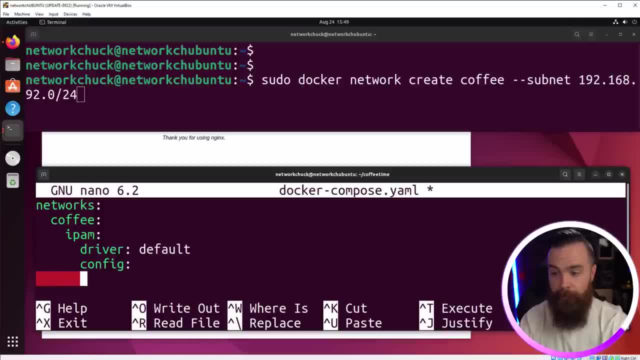 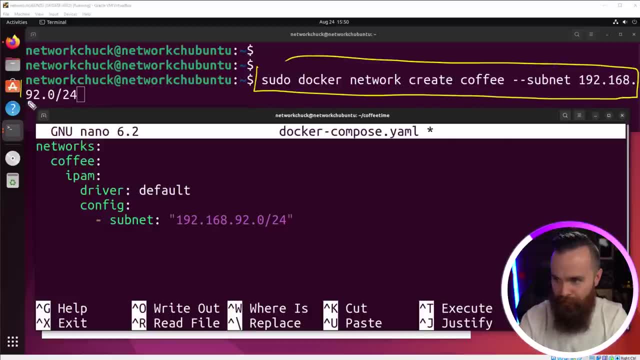 tab tab. We'll do some config colon, enter tab, tab, tab tab, And then we'll specify Our subnet inside double quotes. So that, right, there is how you take that Docker command. And yeah, there's some leftover here on the side. Sorry, you guys forgot about you. That's how. 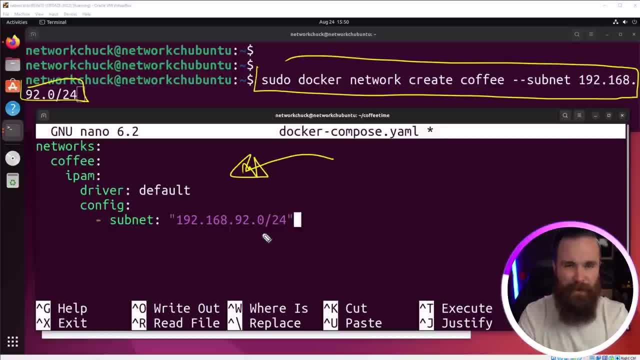 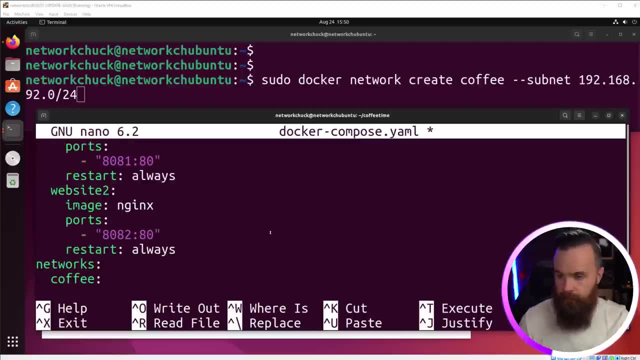 you take that command and convert it into Docker, compose, YAML. Not too bad, Actually, you just have to kind of know it. And then, finally, one more thing: What do you say? We throw one of those containers inside that network? Cuz, right now it won't happen. So let's take website too, Just. 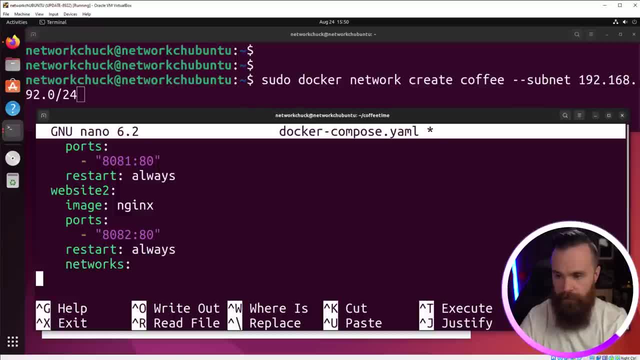 under his restart. I'll add networks colon, enter tab, tab, tab. I'll specify the network coffee And then his IPV four underscore address: Nine, two, one, six, eight, What was that? network 40. Yeah, Or 92,, 92. We'll do dot like 21.. So now, 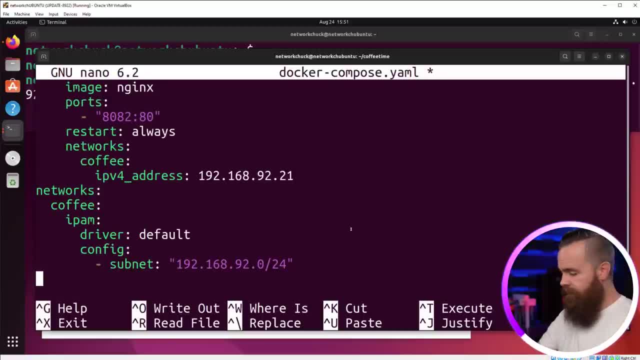 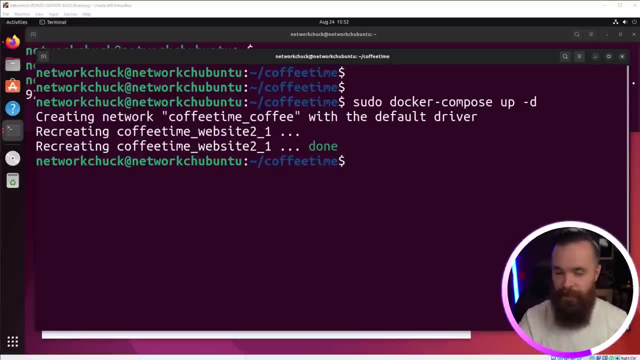 with our compose file, we're creating two containers, one network. Let's save it and test it out. Control X, Y- enter to save Docker. compose up dash D. let's watch the magic happen. That was fast. Now notice something here. We already had our composed file up and running. 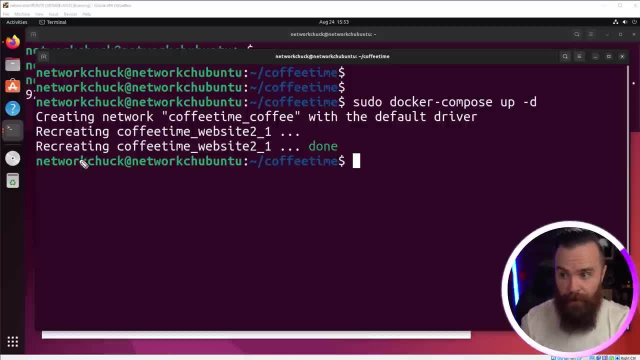 but here, when we changed the file and we ran the Docker compose up command once more, it just updated what we changed. It created that new network and it recreated website too. Let's take a look. We'll do Docker DPS- There they are. We'll do a Docker network LS. There's our two compose networks. 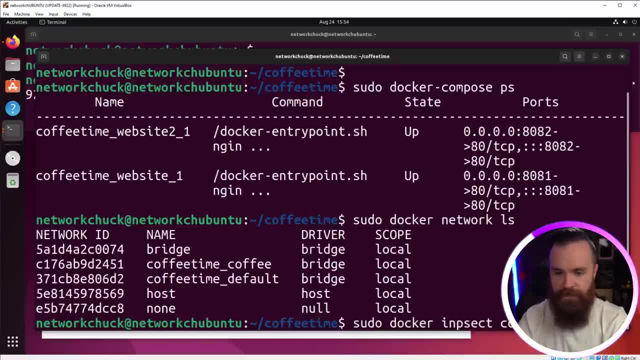 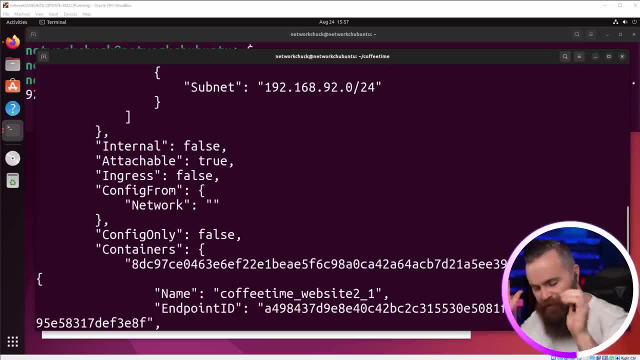 one by default, one we specified. And then if we inspect our new network- Docker inspect, if I spell it right- I can see that container inside right there with the IP address we configured. Okay, cool, So we've done two containers and a network. 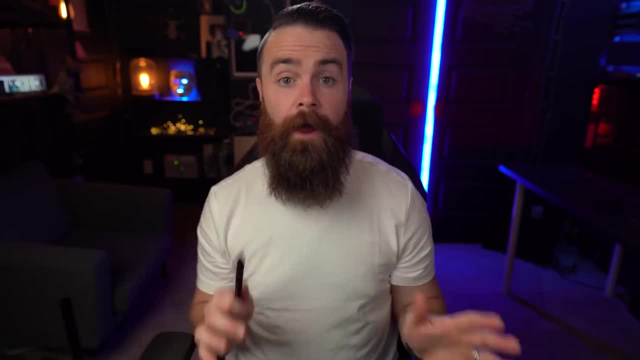 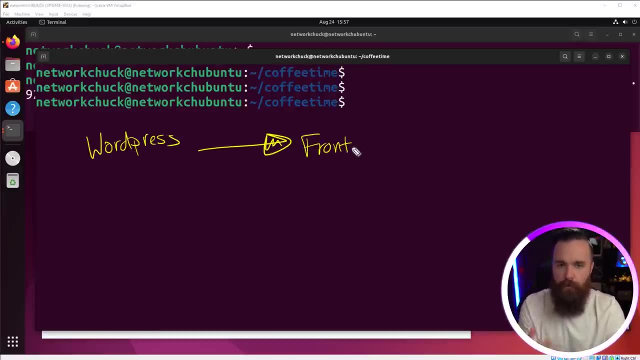 but what do you say? We get just a little bit crazier, and this will uncover the true power of Docker compose, because our next task- I'm gonna clear this out for you- We're gonna deploy WordPress with Docker compose. Now, here's why you would wanna use compose with WordPress, WordPress. 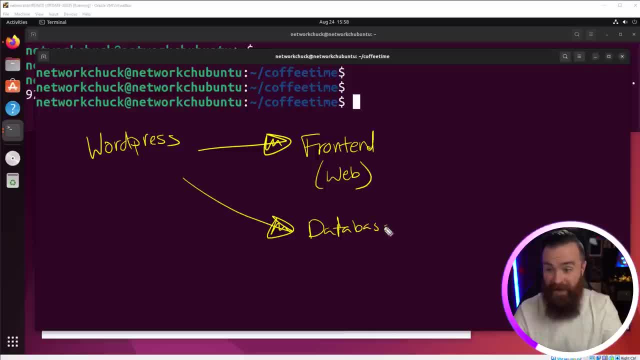 has two main components. It has a front end website or a front end server, and it has a my SQL database. and in a Docker deployment that'll be two separate containers And this will be a bit different because there's something special that we'll have to do to connect these two. 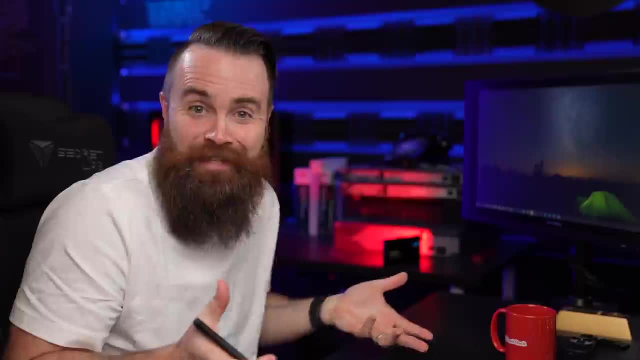 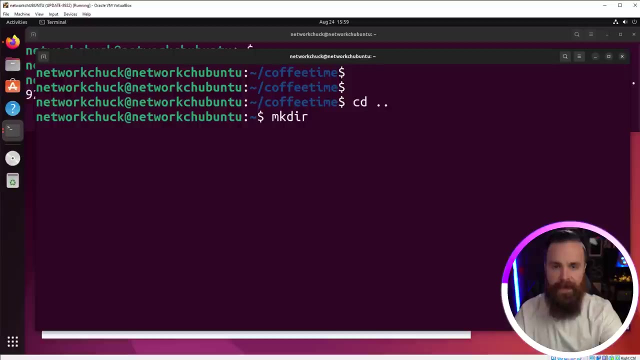 guys to make them kind of well connect and work. Let's try it real quick. So actually, let's go ahead and make a new, brand new compose file. So let's CD dot dot to get out of that directory And let's make a new one, M K D I R WordPress. Let's jump in there. Nano Docker, compose dot, YAML. 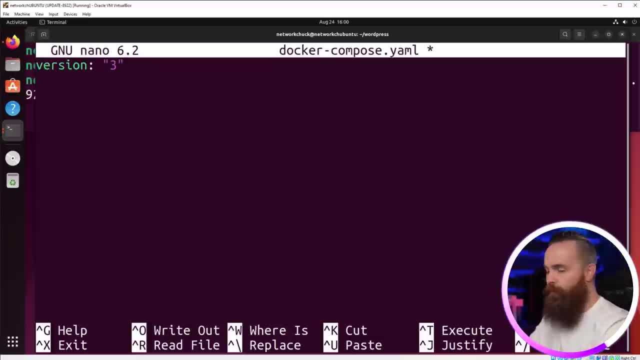 We are in now. same story as before. We'll define our version- Good old three- And we'll start with our services defining our two containers we need for WordPress. First, we'll start with WordPress. We'll call him WordPress. 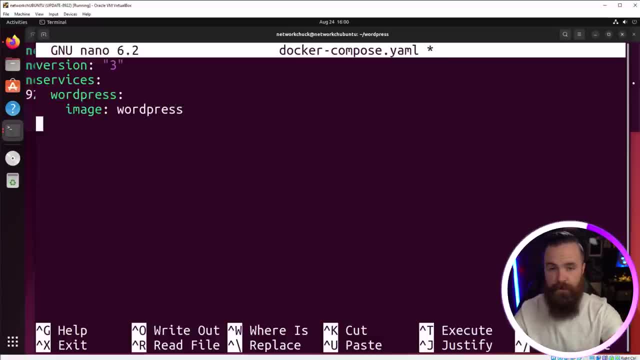 And for our image, we'll simply pull the WordPress image from Docker hub for ports. We'll map port 80 to 80- 80 on our machine, Actually. No, we need to do something else, Don't we? Let's do like 80: 89,. 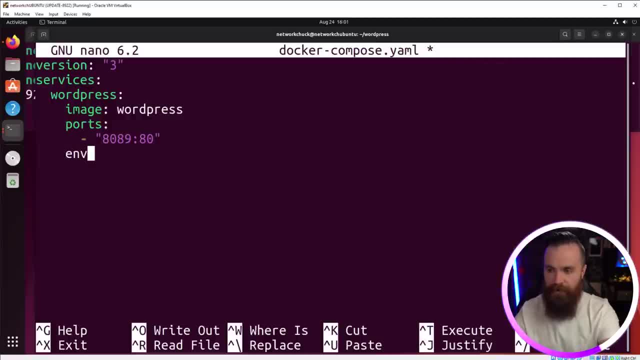 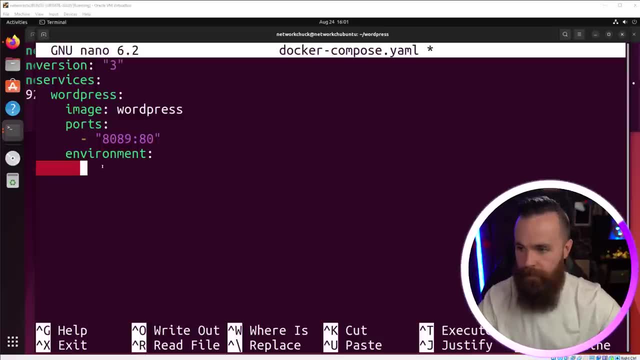 because I forgot where we were. And the next is something interesting. We're gonna have something called environment, And here we'll put specific parameters that are specific to WordPress inside the WordPress environment. Let me go ahead and paste a few right here You can copy. 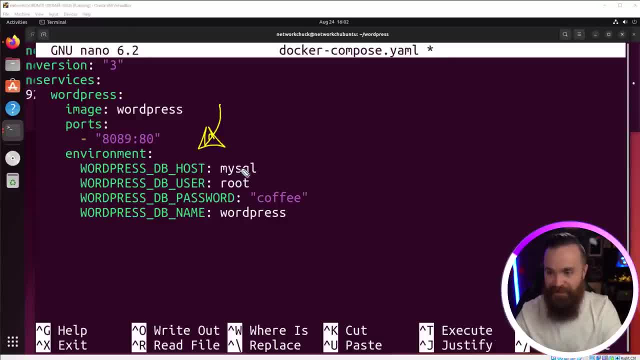 copy the code from below as well. Noticing: here we have things that are specific to WordPress, like all the database info. We can pass those environment variables into WordPress as we're creating a container, And pretty much every one of these are referencing what we're about to do. 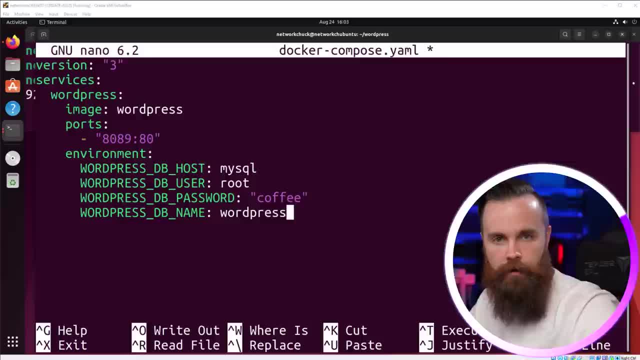 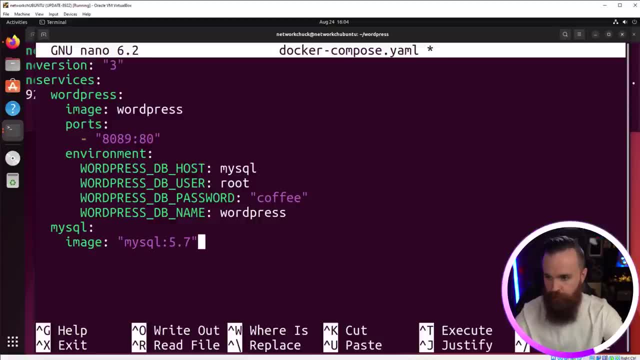 with a SQL server or a my SQL server- sorry, my SQL. So we'll go ahead and add our my SQL server. We'll call that service My SQL. the image will be my SQL, colon 5.7.. And I'll put that: 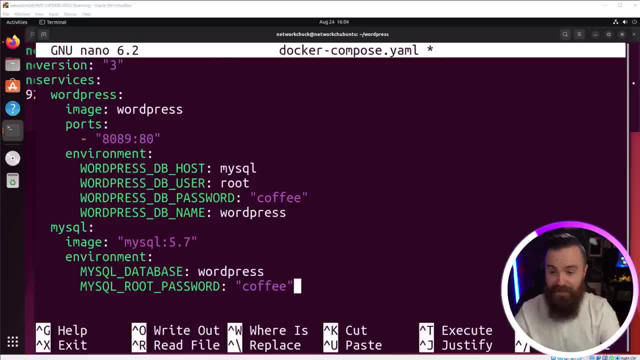 between quotes, And then we'll also do some environment variables for him. So now we're seeing that WordPress is matching the SQL service as his database word as coffee and the database name as WordPress. Now a couple of cool things we can do with. 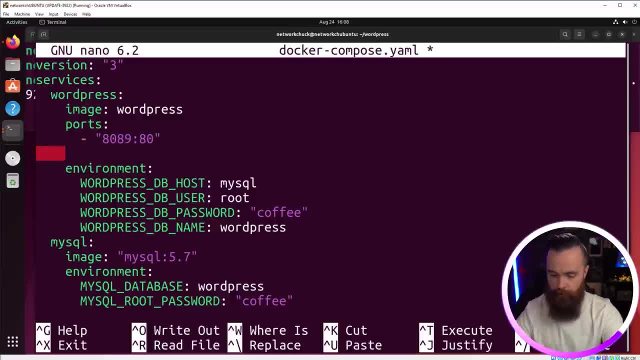 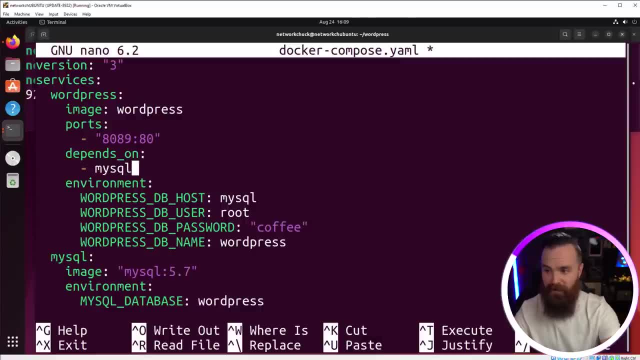 containers and how they interact. first, up here in WordPress, let's add another parameter and we'll call this: depends underscore on colon. I want to enter a couple tabs and we'll tell it to depend on my SQL. And this is cool, Cause what this will do is tell Docker: compose Hey. 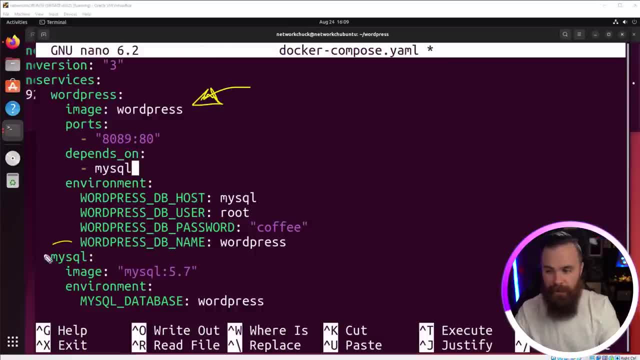 before you make this WordPress container, even if he is the first guy up here, make sure you make the my SQL guy first, because WordPress depends on him, So you can tell him to do that. That's kind of neat. So don't make him until you've made him. And one more cool thing. 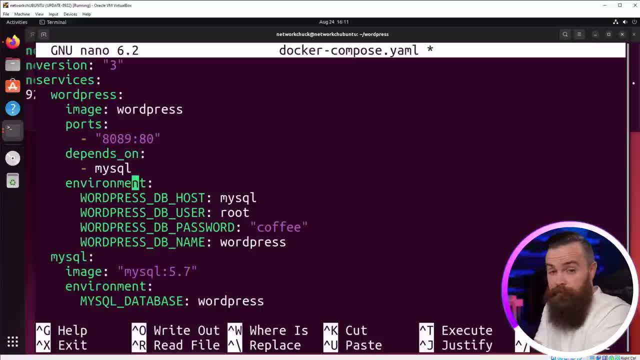 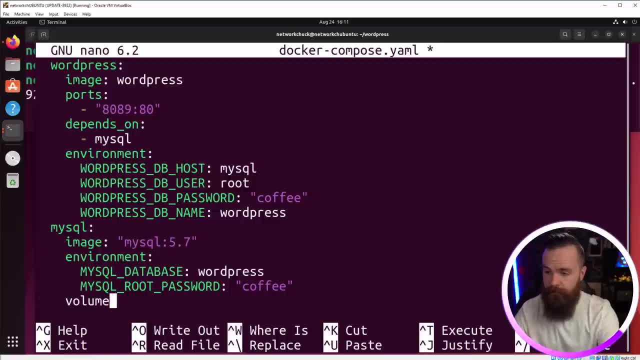 you might wanna add to your WordPress deployment, cuz you could legit just run your WordPress website inside Docker like this. but here on the my SQL container let's add one more section and we'll call this volumes and Docker. volumes allow us to map a Docker directory to a directory on our system, on the. 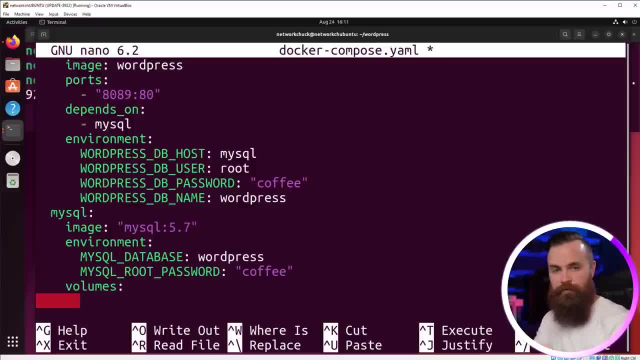 host system. That way, if the Docker container ever gets blown up, dies or restart it, delete it. whatever that directory, the data still exists on the host, which is kind of important for a you know database. So we can simply map it like this, telling it: Hey, in this current directory. 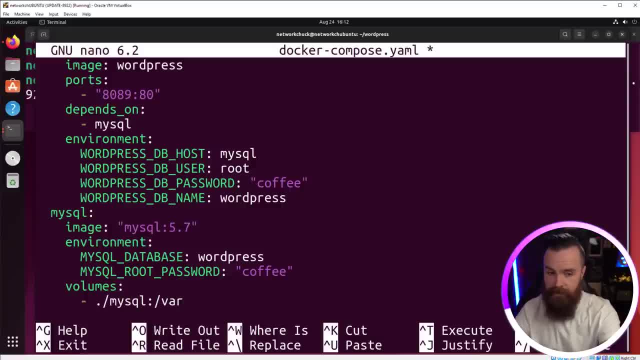 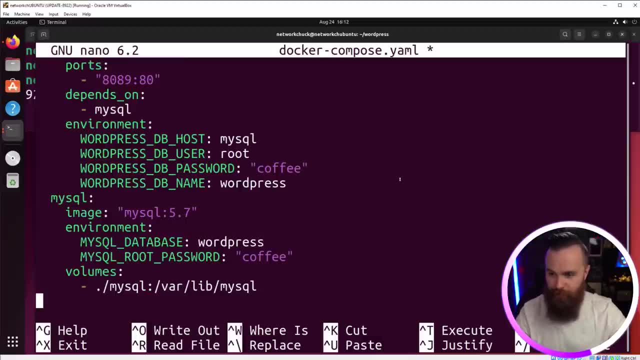 go ahead and create a volume called my SQL And map that to inside the container VAR lib, my SQL, which is what my SQL cares about. Now this will work beautifully, but I do wanna go through the trouble of adding a network, If you. 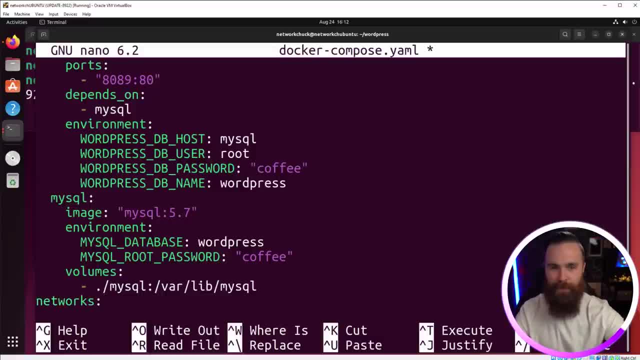 know how to do that. if you remember how to do that, go ahead and do it right now, Cause I don't want Docker creating that for me. I wanna do it myself. Call it, Oh yeah, Then I'll add those containers to the network. So there's our completed Docker compose file right here. 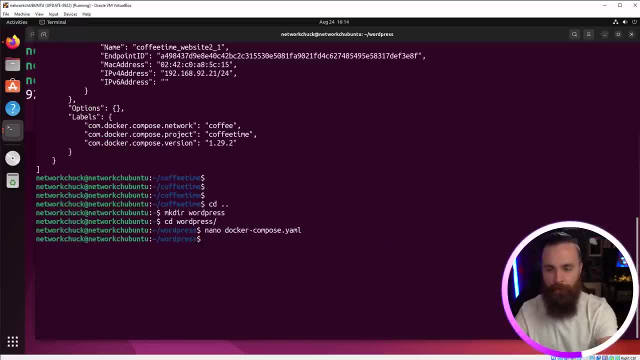 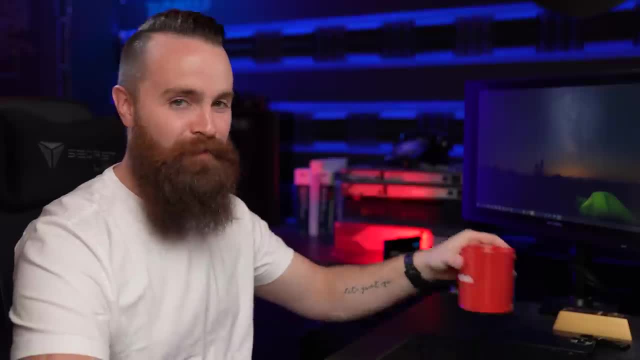 Isn't she pretty. So let's control X, Y, enter to save, And let's bring that bad boy up. Docker, compose up dash D. it's gonna download all the things it needs for WordPress and my SQL. It'll do a quick coffee break. This feels like magic when it's doing that. I love it And just like. 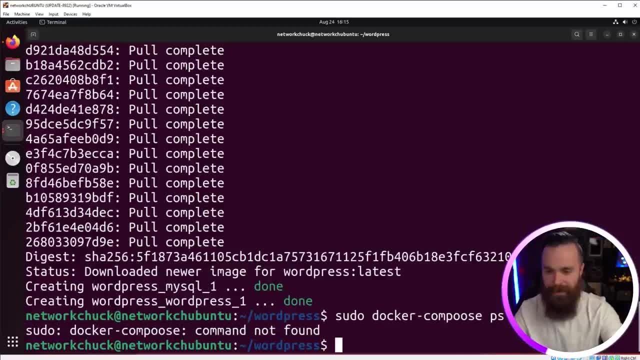 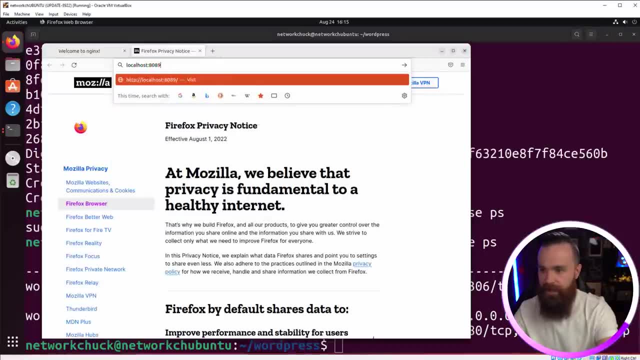 that we get a WordPress website running. I'll do a little Docker: compose PS, not compoose, compose PS. There they are, Let's see if we can get to it. Local host: port 80: 89.. Yes, WordPress website. 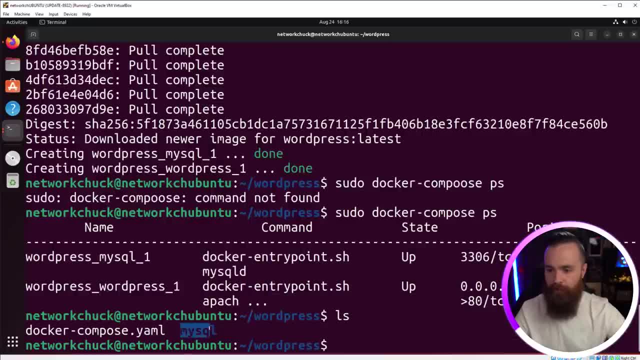 That's so cool. And also notice, if I do an LS right here, there's that my SQL folder. That's where my SQL is mapped. I jump in there. There's all the my SQL goodies. So if I were to do a, 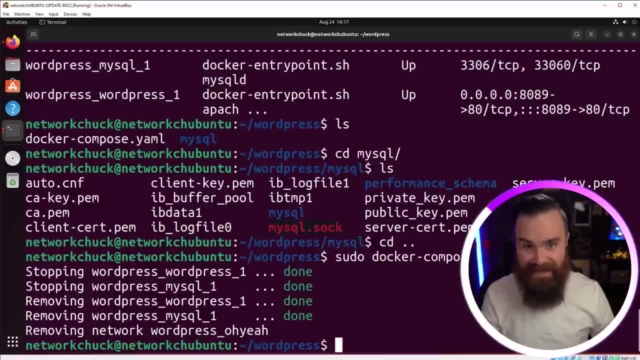 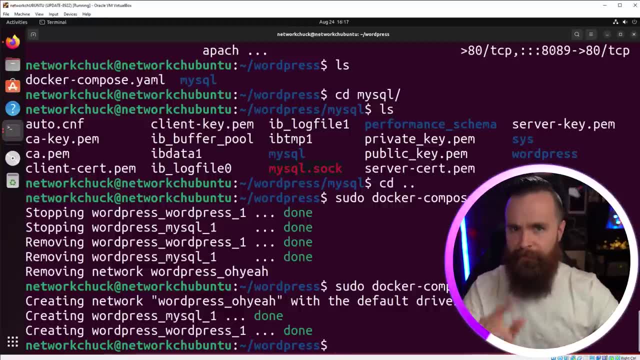 pseudo Docker: compose down, Okay Down, and delete it. I still have my database intact, which means bringing it back up. Yeah, It's creating brand new things, but my SQL is still in mapping to that same database file And, if I refresh the page, same stinking website. that's pretty cool. Now, of course, you can deploy. 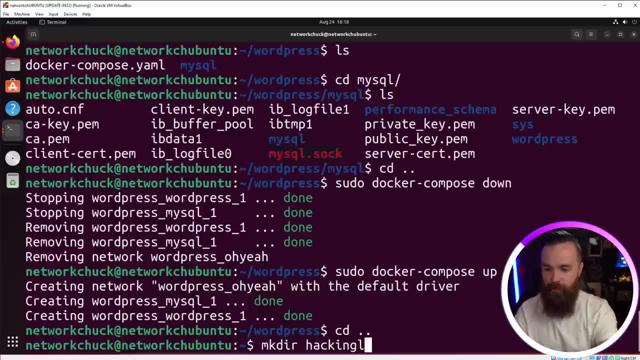 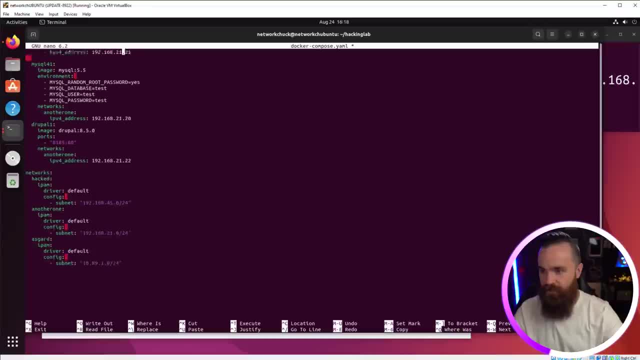 that lab I showed you earlier. So if I do that right now I'll see hacking lab, my new directory. I'll start my Docker compose file And I'll just paste all that in there. It's a lot, but you'll notice that it looks familiar. We've already talked about a lot of this. It's just a. 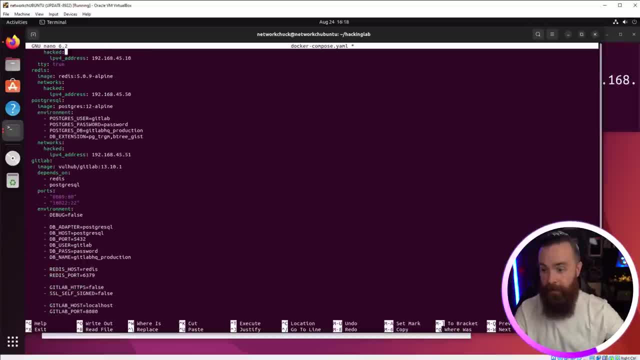 bunch of networks and a bunch of containers all connected together in various ways. by the way, Yes, All of these are vulnerable containers from a place called vol hub, not vol hub, vol hub. They basically turn vol hub uh virtual machines into containers. So shout out to them, I'll put. 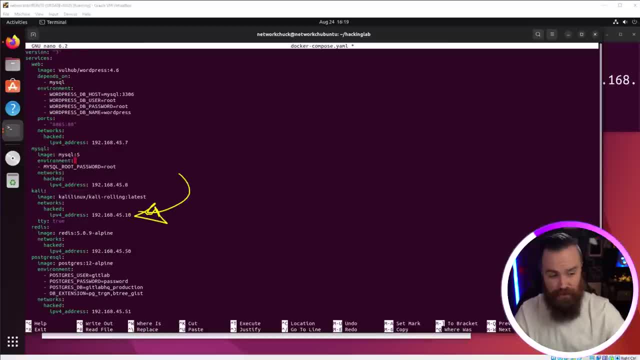 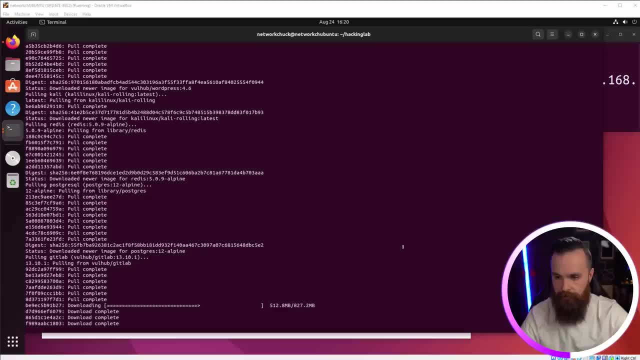 a GitHub link below, And of course also right here I have my Cali Linux machine, which is cool because once I launched this, go ahead and do it right now. that's gonna take a minute, Cause that's download all those uh container images. So while that's downloading, 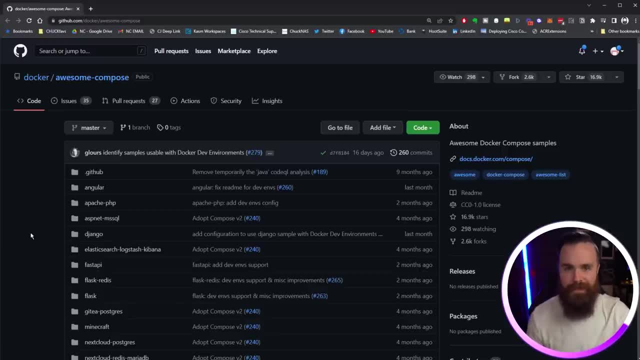 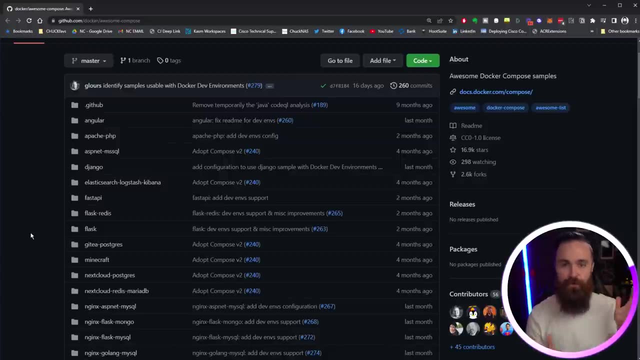 it might take a minute for you, It's taking a minute for me. Here's some Docker compose inspiration Cause again, companies mainly use Docker compose to deploy their apps, Cause they kind of package them all together, make sure they're connected the right way, So things like.